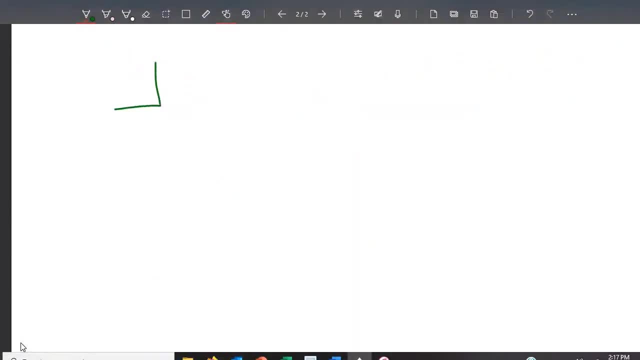 sure you remember. All right, so we bring down the coefficients, so it's going to be 1, negative 2, negative 11, and 2. The number that goes here: remember when it gives me this information, when it's written like this: 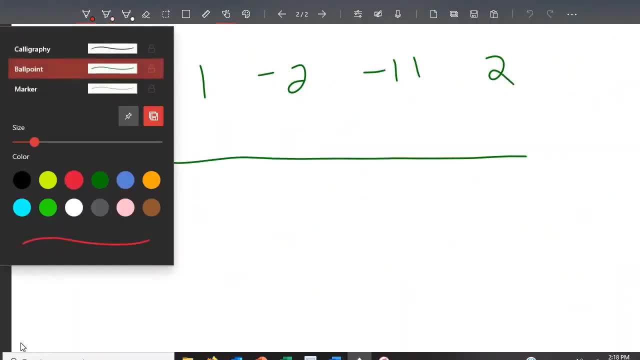 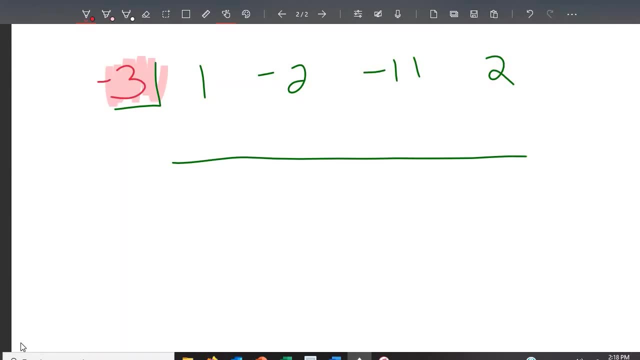 that's the number that goes in the little half box. It's giving me the number to put in here already. Now let's do the synthetic: Bring down the 1.. Now, since I'm told it's a root, I should get a zero right here. 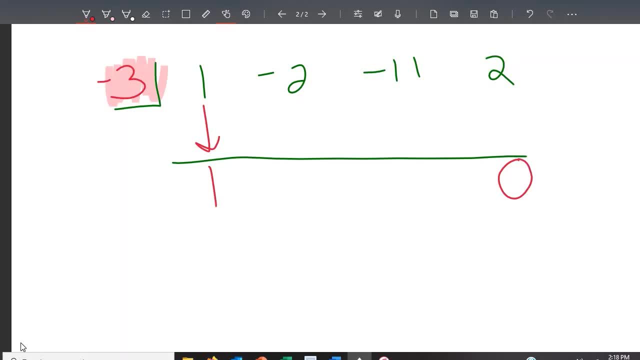 If I don't get a zero, then this book is wrong. So there we go. So multiply negative 3 times 1 is negative 3.. Add the two numbers Negative, 1, negative. 5 times negative, 3 is positive 15.. 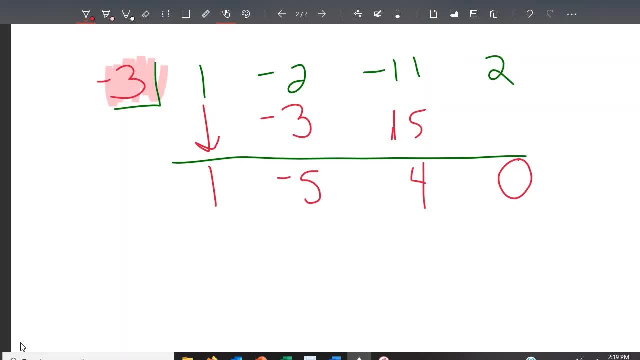 I'll get 4.. Hold on, I must have wrote it wrong. This should be a 12, not a 2.. I wrote it down wrong. That's a 12, right there. Okay. so 4 times negative 3 is negative 12,. 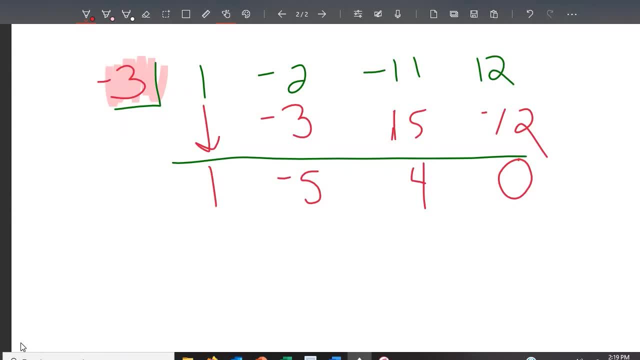 which gives me my zero. So we bring down the numbers, the coefficients, and put them back in front of the variable. Set it equal to zero, Then we factor and solve for the other two roots, or zeros, or whatever you want to call them. 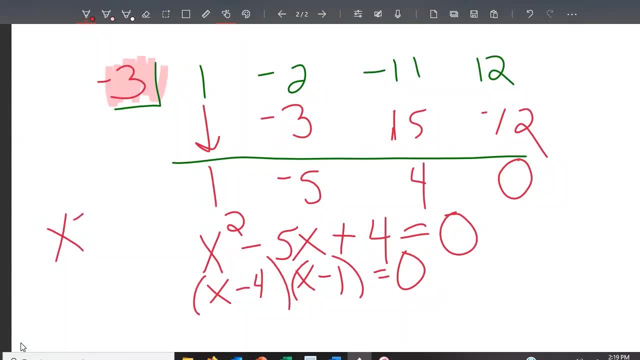 So, when we solve this, when x minus 4, we'll get x to be positive 4.. The x minus 1, x will be positive 4. So we'll get x to be positive 9.. These are my three solutions, also called roots, also called zeros. 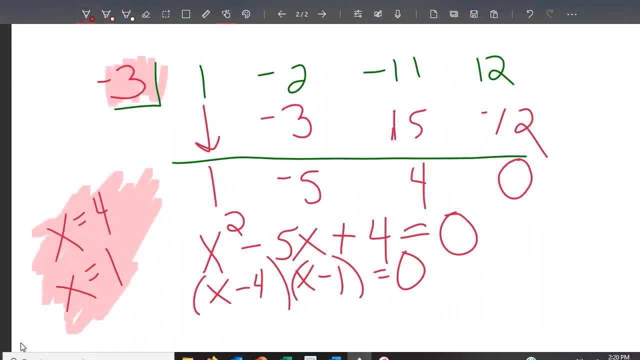 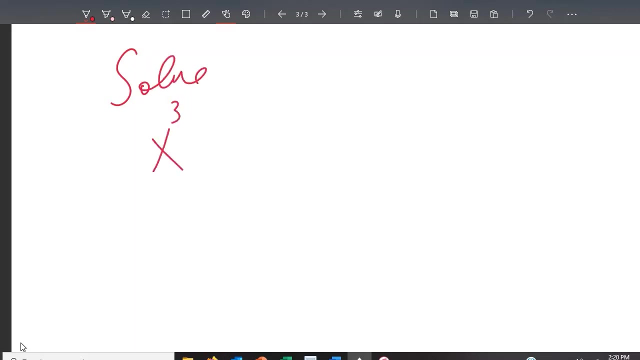 Now, in this example, we were told what to put right here. Well, that's good. I need to know that in order to do these problems. Now suppose, though, I gave you this, I said: solve x cubed minus 2x squared. 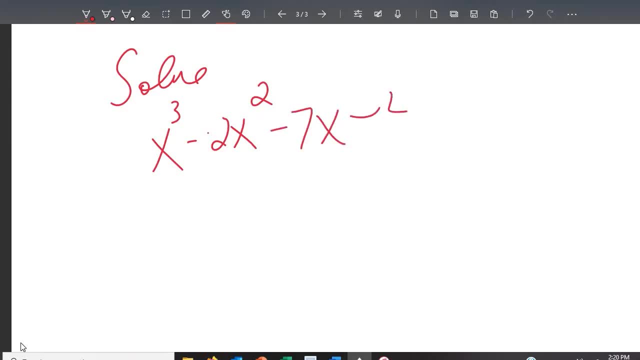 minus 7x plus no minus 4 equals zero, And that's all I tell you. I'm not told something. well, where is a root? where is the info about a root? yeah, that's the problem in this section: you're not told what the root is. so what we have to do, 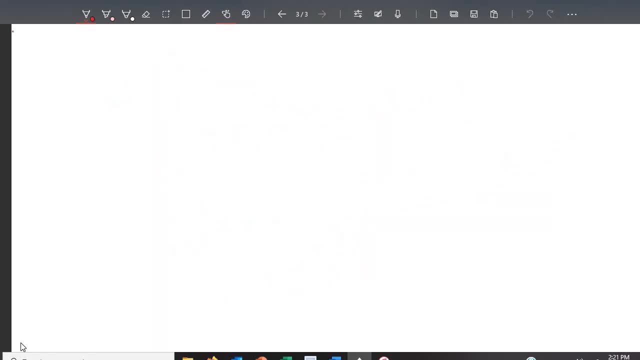 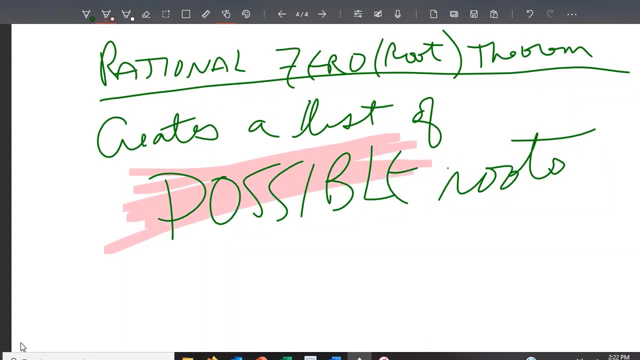 is something called the rational zero theorem or the rational root theorem. what the rational root theorem does? it creates a list of possible roots and highlight that possible. now this is possible. that's doesn't mean they are. it means this could be. now our lists are going to be. 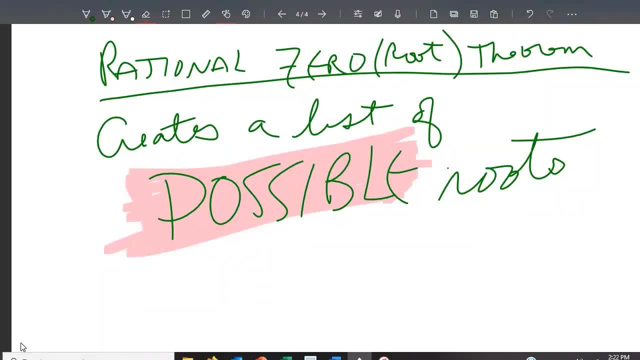 some of them are going to be kind of long. I might have 16 possible answers. I might have four possible answers. I could have, you know, 30 something possible answers. this is where it gets very tedious and very. I don't say it's not complicated, it's just tedious. and once we miss this route we're going to use. 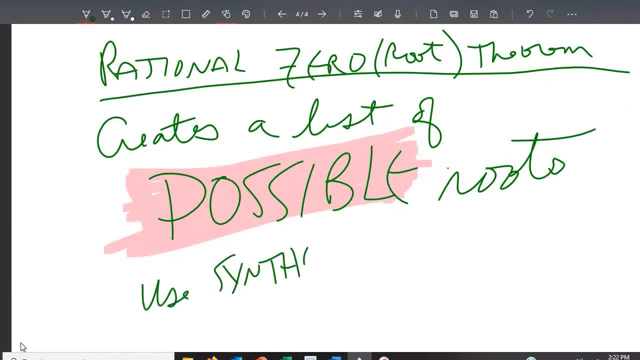 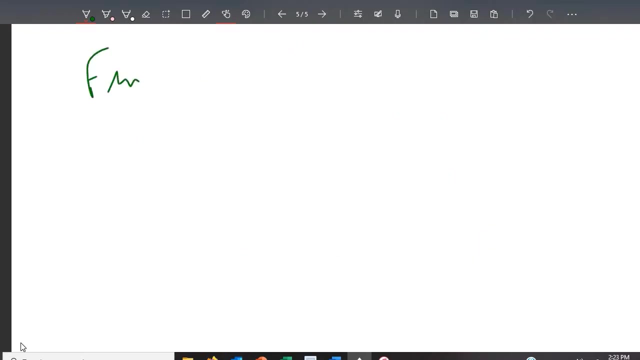 synthetic to find a zero. so instead of us being told up front, we got to go find, find it ourselves now, in order to find the roots, find possible roots you do is you list all the factors of the constant and you divide them by all the factors P of the first number. so you have to go create a list based on the factors of. 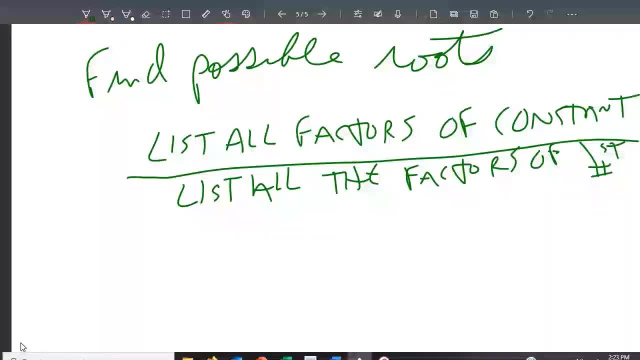 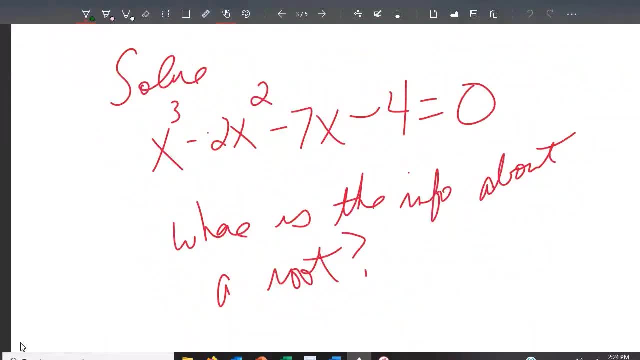 the first number and the factors of the last month. now, what was this example I had over here, alright, so I want to take this one. now it's a four. it's gonna be a fairly simple one, so I want to list all the possible factors, I mean find the possible roots for that previous. 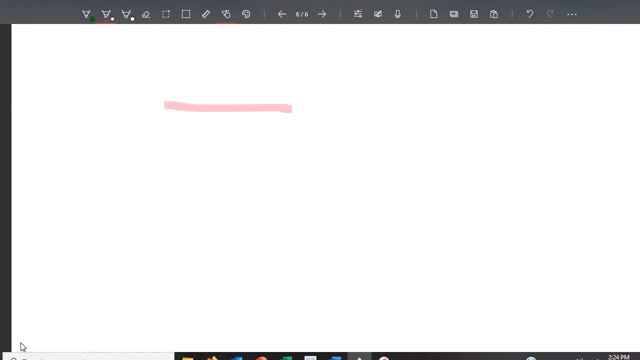 previous example. so we're going to create a fraction. when you're listing the factors, you must put a plus or minus in front of each factor, so the factors of last number go up top, The factors of the first number go in the bottom. and it was just a 1,, so that's good. 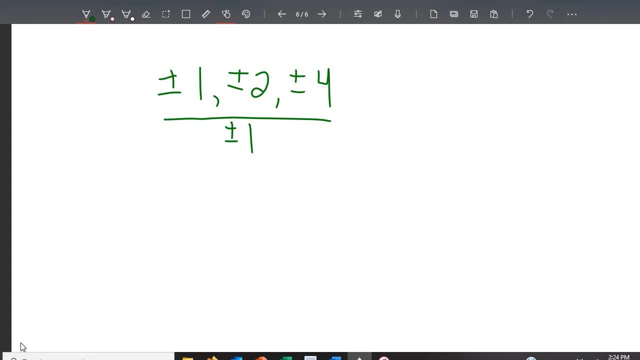 Then you take each number in the bottom and you divide it into each number in the top. In this case, we're just dividing them by 1, so this is what we end up with Now. I want you to notice I have 6 possible roots because of that plus or minus. 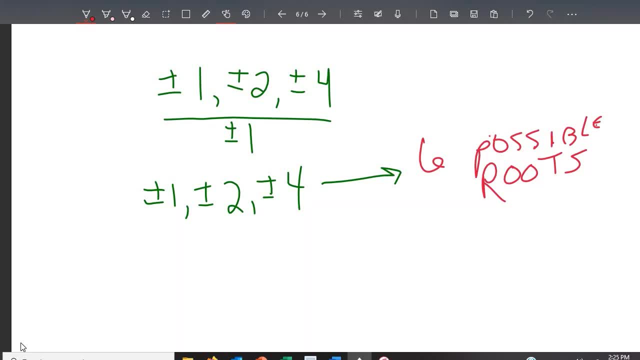 What I would do if I wanted to solve this equation. I would have to take each one separately, use synthetic division and then do this until I get to the bottom. I find a remainder of 0. Before I do that, I want to practice finding these possible roots. 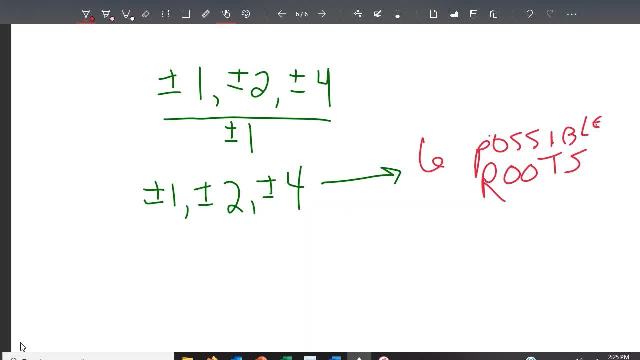 Let's do this one. Let's say I want to list all the possible roots. List all possible roots. The number of the root is drawn out of 2x cubed, or the function 2x cubed minus 3x, squared minus 11x plus 6.. 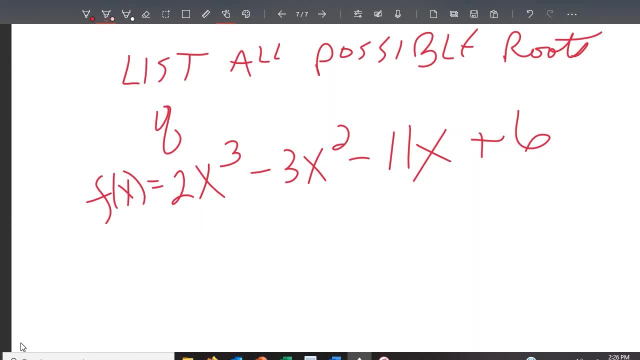 Now I'm only looking at the last number and the function, So that's something that I'm going to do later. So that's something that I'm is just trying to do. We just need this to be there: How many N in the sum of these individuals? Who want them to join in as we go. of course They can be these by taking the automatically counting down the variables instead of theICE 別的WHERE. It doesn't matter how many numbers they need to go top and에서, I want them to be together. 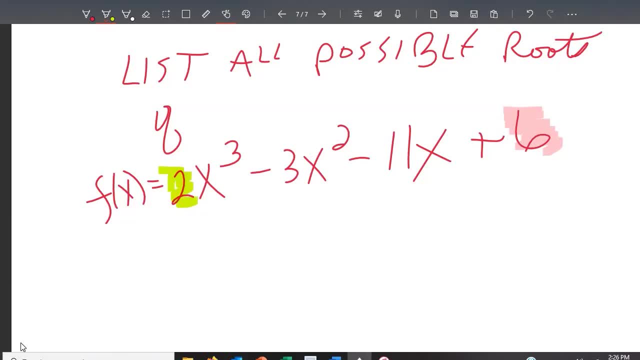 first number. I don't care anything about the negative 3 and the negative 11.. You've got to remember to put the factors of 6, the factors of the last number over the factors of 2.. So the last number goes on top and the first number goes on the bottom. Now let's list all the. 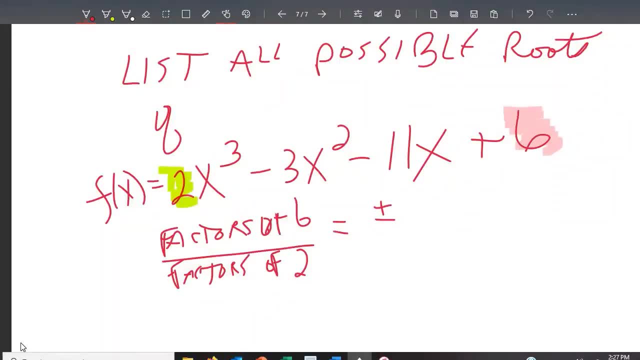 factors of 6.. Now make sure you put plus or minus in front of each one: Plus or minus 2,, plus or minus, plus or minus 3,, plus or minus 6.. Then you're going to have in the bottom plus or minus 1,. 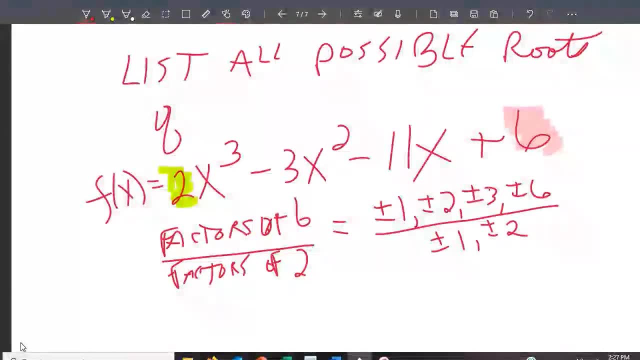 plus or minus 2.. Now here's where you've got to pay attention. I'm going to write it out the long way, then we can simplify. You're going to take each number in the top and divide it by each number in the bottom separately, So it will look like this: 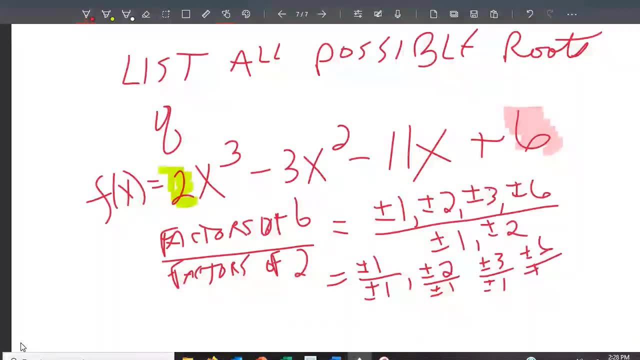 Alright, So that's doing the ones. You turn around and you'd say: OK, plus or minus 1 divided by plus or minus 2, plus or minus 2 divided by plus or minus 2,. plus or minus 3 divided by plus or minus 2,. plus or minus 6 divided by plus or minus 2,. 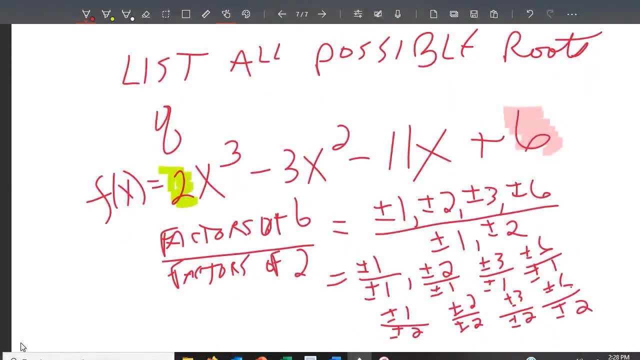 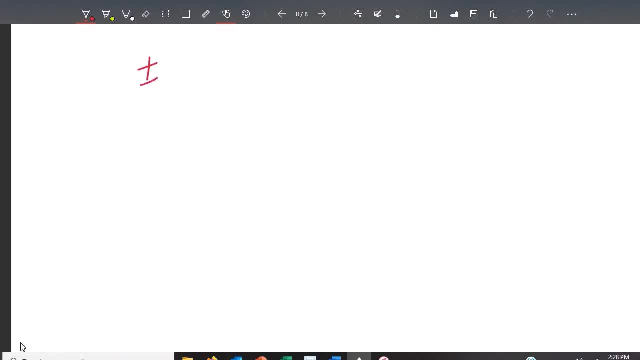 Now you're going to go simplify these. I'm going to come over here to the next slide. So we're going to get: 1 divided by 1 is 1, 2 divided by 1,, 3 divided by 1, and 4 divided by. I mean 4, 6 divided by 1.. 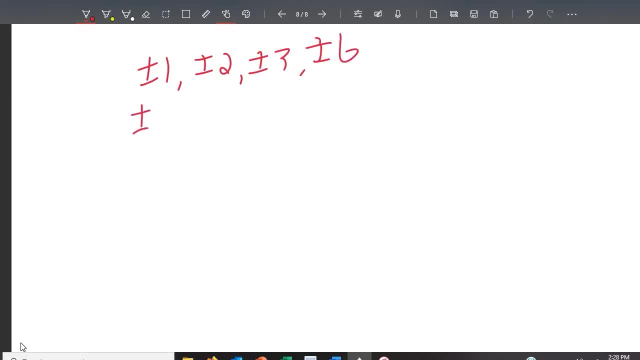 Then we're going to have: 1 divided by 2 is 1 half. 2 divided by 2 is 1, which we already have. then we're going to have 3 divided by 2, then we're going to have 6 divided by 2, which is 3,, which we already have. 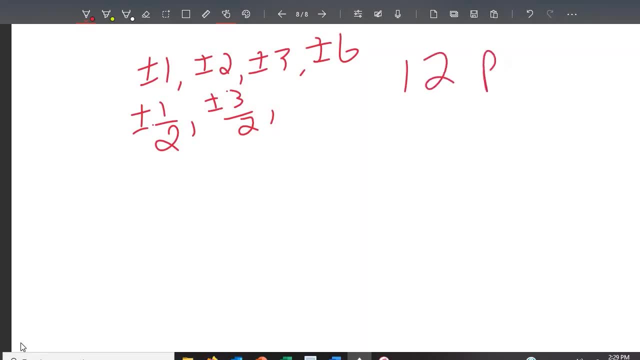 Now notice I got 12 possible Roots. It is possible none of those work. I'm going to have them where they work, but we have to be able to create this list. Let's say I had I don't know. let's say my function is we'll do 4x squared, I mean 4x cubed. 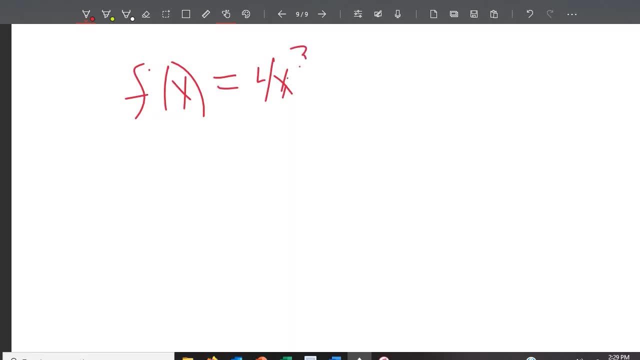 7x squared plus 3x plus. oh, let's do 15.. Okay, so we would take all the factors of 15, the bottom, I mean the last number in the top, Then in the bottom we would put all the factors of 4.. 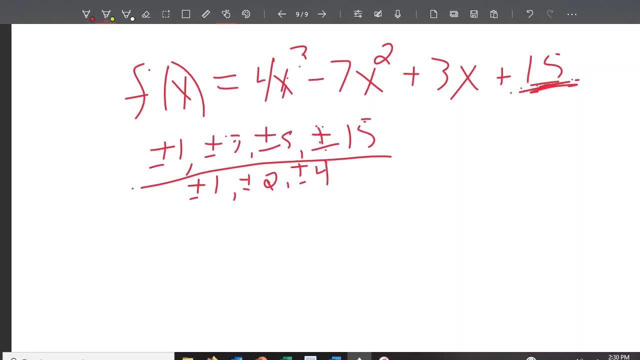 Now, first thing I'm going to do is divide the top numbers by 1.. When I divide the top numbers by 1, we'll get plus or minus 1, plus or minus 3, plus or minus 5,, plus or minus 15.. 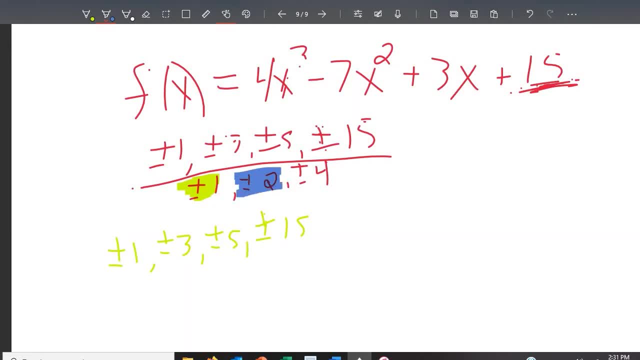 I'm going to take the top and divide everything by 2.. So we'll have, oops, Plus or minus 1 half, plus or minus 3 halves, plus or minus 5 halves. plus or minus 15 halves. 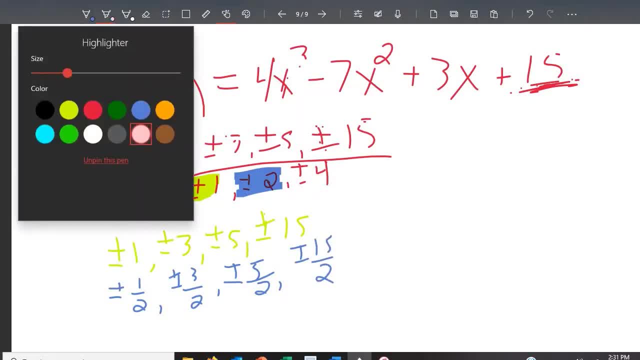 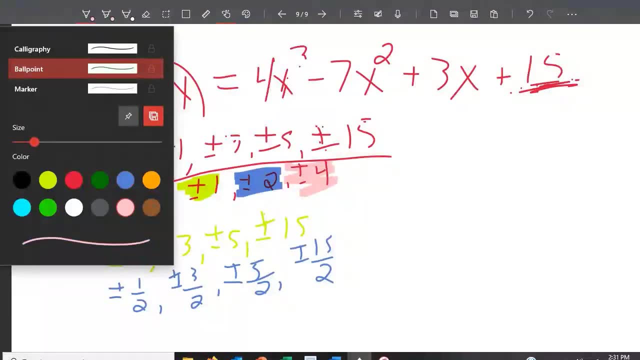 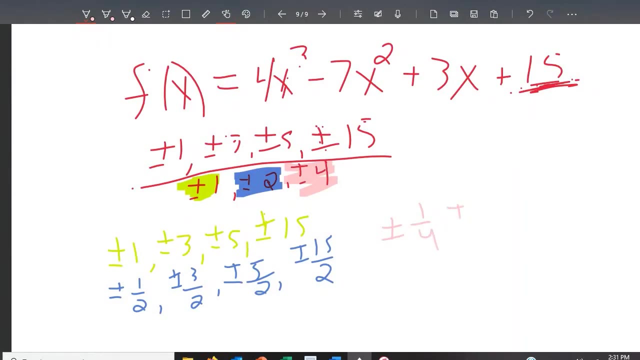 Then I'm going to take the 4 and divide it into everything in the top, So we'll have plus or minus 1 half. Plus or minus 1 fourth. plus or minus 3 fourths. plus or minus 5 fourths. plus or minus 15 fourths. 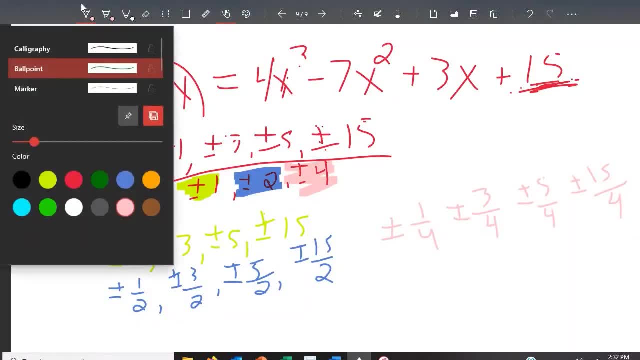 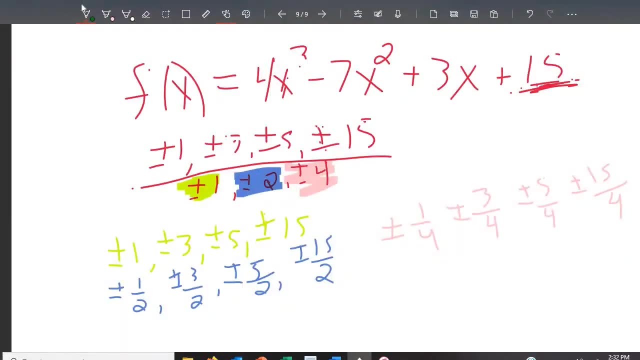 Now, this is an extreme problem. There are- let's see, let's see- 24 possible roots. Our goal is to use synthetic division and these numbers and try to find one that gives me 0 at the end. This is where it gets very tedious. 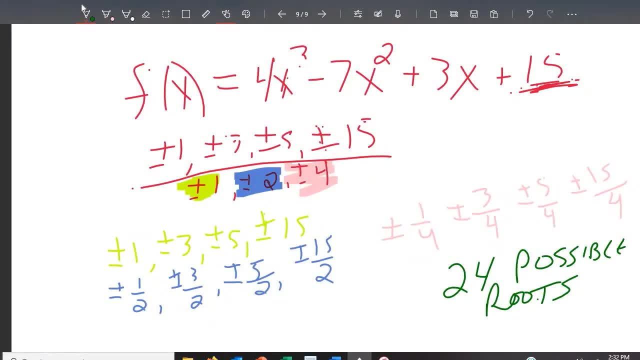 You would have to take each one separate. You don't know which one is going to work. You have to do them separate until you find a 0.. Now I would not have one this extreme on the quiz, but I do want to show you how you can go about this. 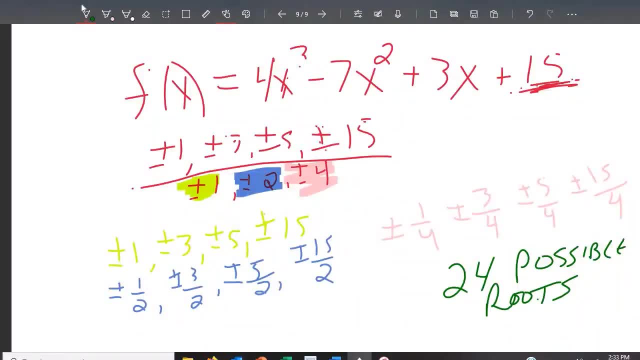 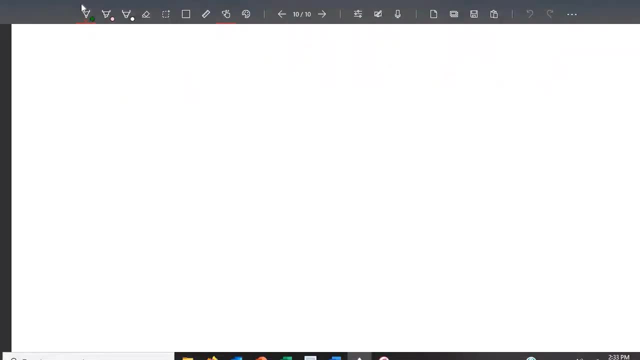 Let's do try to find a good one here. Let's start with so I want to solve x cubed Minus 2x squared plus 7x minus 4.. I already did this one earlier: Minus 4 equals 0.. 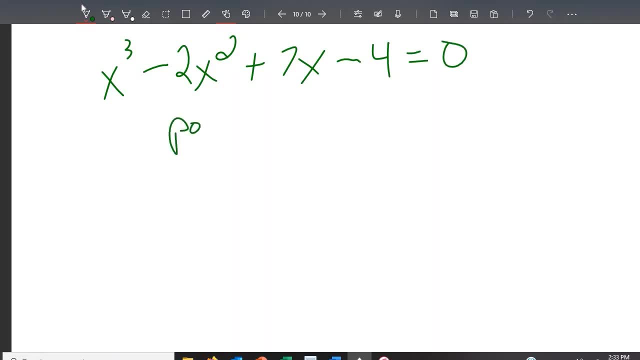 Alright, First thing you do is list out your possible roots, and I did this one earlier. The possible roots are: plus or minus 1,, plus or minus 2,, plus or minus 4.. And you set up your synthetic division. Whoops, that should be a minus 7.. 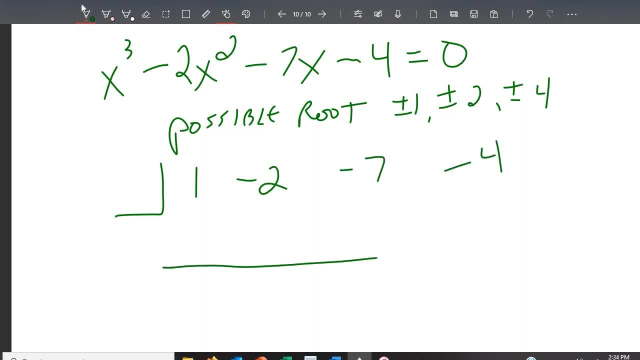 And that should be a minus 4.. And you know, you set it up just like normal, But this time I don't know which number works, so we have to go check them, Literally check them. So I'm going to start with positive 1.. 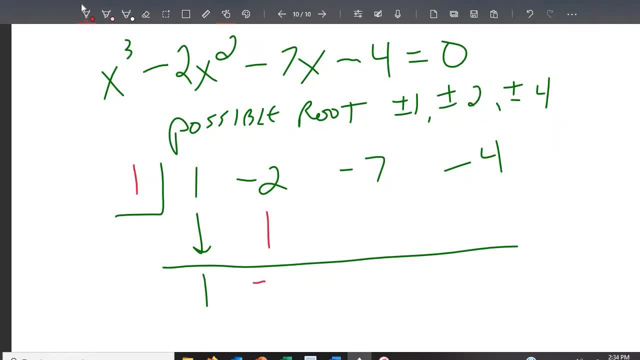 1 times 1.. 1 is 1.. Combine that together, we'll get negative 1.. Negative 1 times 1 is negative 1. Combine that together, we'll get negative 8.. Negative 8 times 1 is negative 8.. 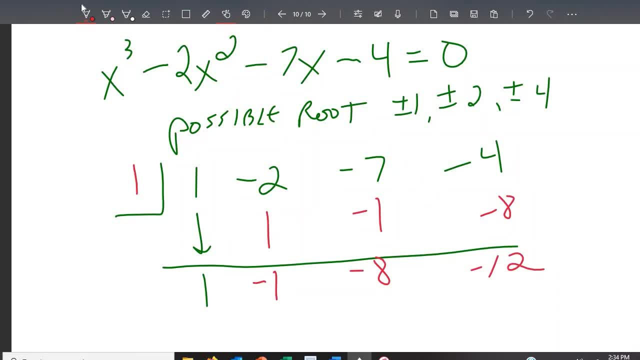 And I get negative 12.. Well, I need a 0 right there where that negative 12 is. So what that means. this positive 1 doesn't work. So then I choose another number out of that list. I usually just start with 1 and work my way down. 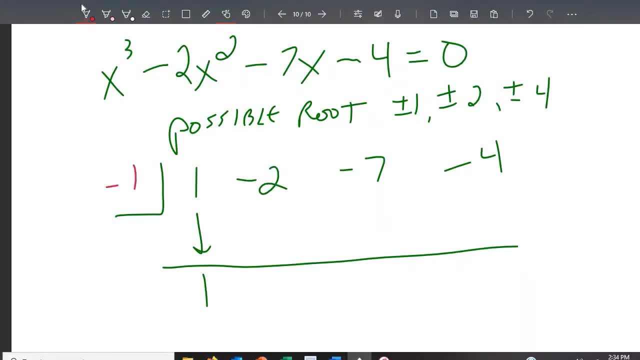 Let's try negative: 1. Well, 1 times negative, 1 is negative. 1. That gives me negative. 3. Negative: 3 times negative: 1 is positive, 3. I get negative. 4. Negative 1 times negative: 4 is positive, 4.. 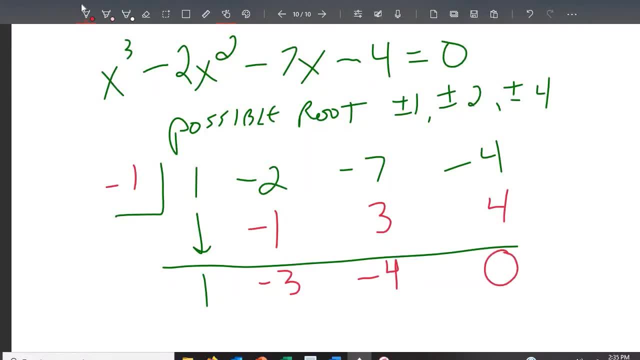 And guess what? I get 0. What that means this is a root, Which is the same thing as a 0. Which is the same thing as my solution. So one of my answers for this problem is: x will be negative 1.. 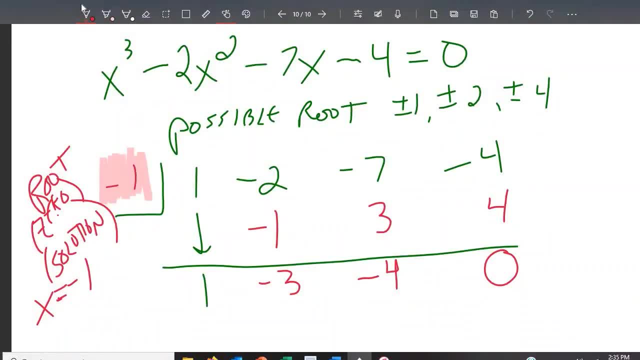 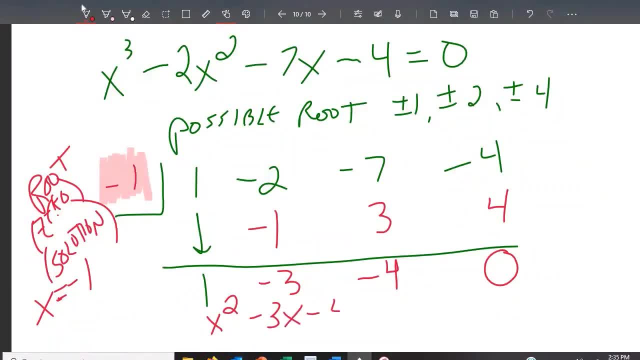 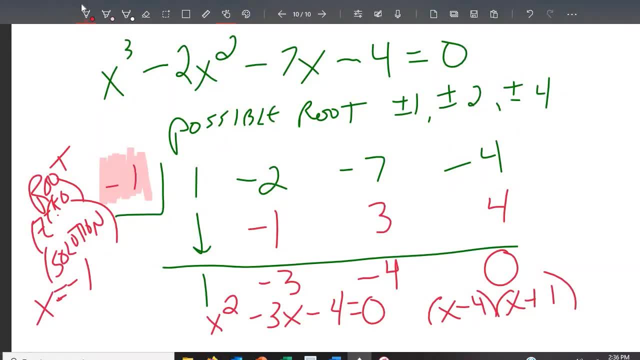 Negative 1.. Negative 1. equals 0. now you know, we already know how to do this. this is going to be x equals 4 and this is going to be x equals negative 1. well, I've already got negative 1, so my other answer is x equals 4. so that's one of my answers. I 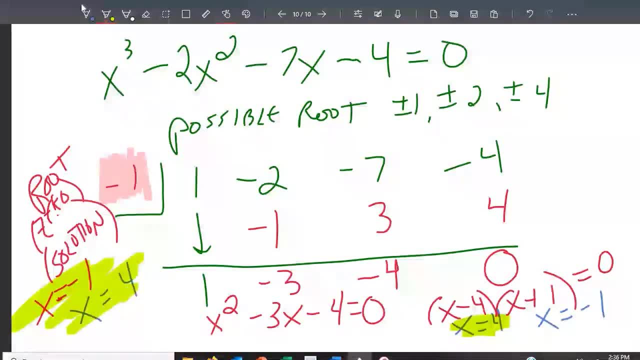 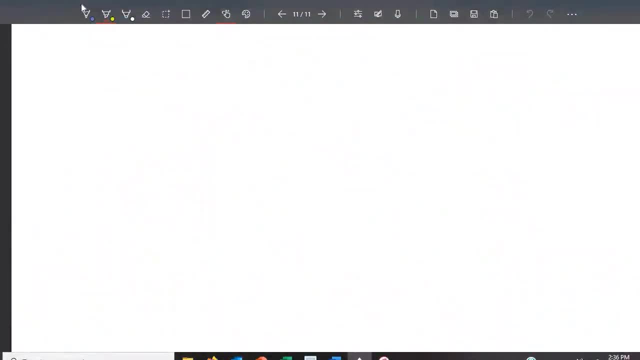 already had, then I already had the negative 1, so this one has two answers. let's do: 6x cubed plus 25x squared, minus 24x plus 5 equals 0. okay, now here comes the possible meaning. you gotta list out your. 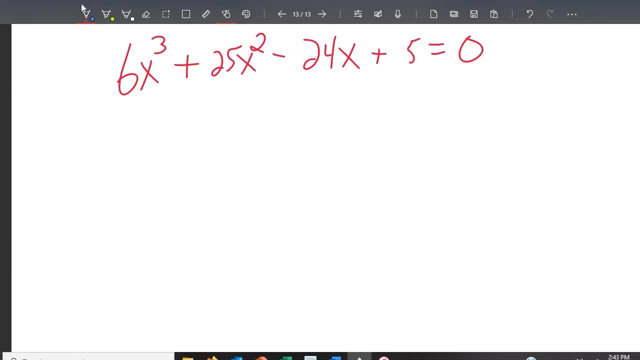 possible roots. there's a question on the final, where it just says list the possible roots. remember, it's always the last number, so it's the factors of the last number divided by all the factors of the first number. you, okay? so we take every number in the top, divide it by one, take every number in the. 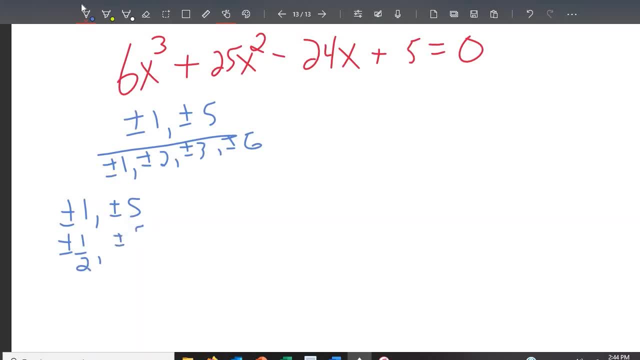 top, divide it by 2, take every number in the top and divide it by 3, take every number in the top and divide it by 6.. Wow, what a mess: 16 possible roots and only 4 of them are whole. 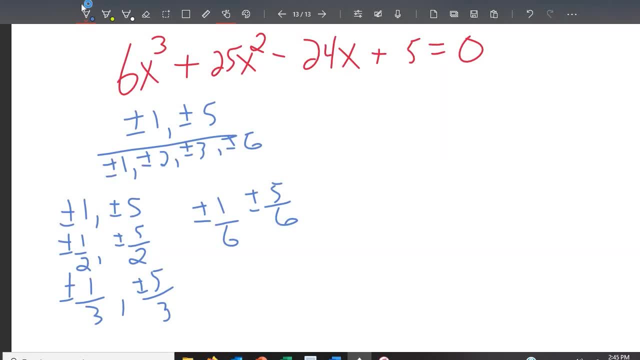 numbers. Let's hope there's a whole number that works, because I don't want to deal with these fractions, but let's just go do the synthetic, see if we can find one that works. I always try to do the whole numbers first and then, if I have to, I'll do the fractions. 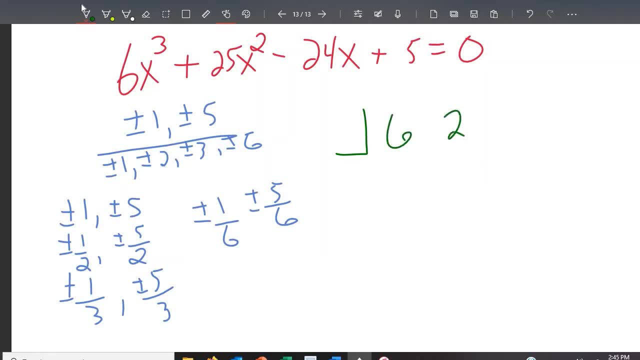 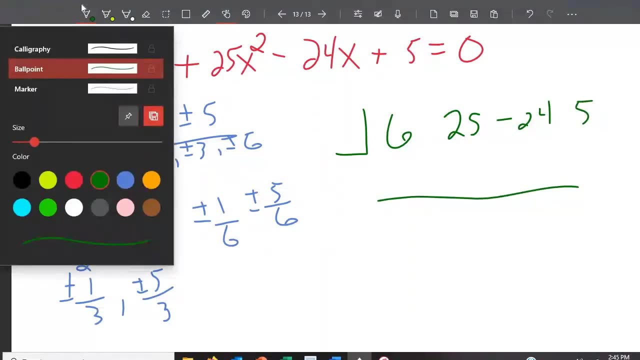 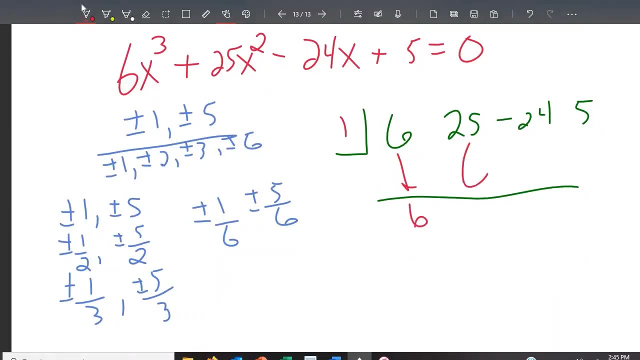 So I'm going to definitely start with the whole numbers. Alright, let's just start with 1.. Again alright, 6 times 1 is 6.. Combine that, we'll get 31.. 31 times 1 is 31. I'll get 7.. 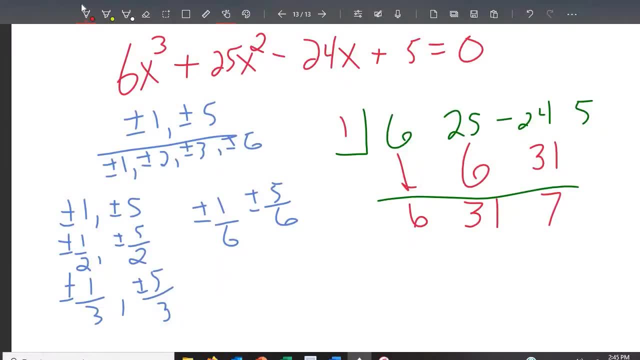 And that's definitely not going to give me a 0.. So start over. Let's try negative 1.. 6 times negative 1 is negative 6. That's going to give me 19.. 19 times negative 1 is negative 19. And that's not. 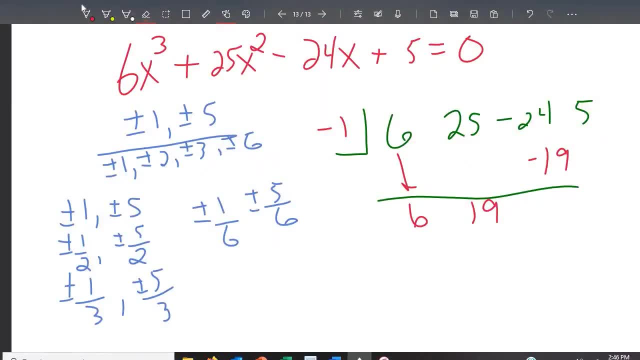 going to work. This is the way it works. sometimes You just have to check 3,, 4,, 5,. uh, you know, let's try 5.. 6 times 5 is 30. Gives me 55.. Whew, I hope you can tell that ain't going to work. 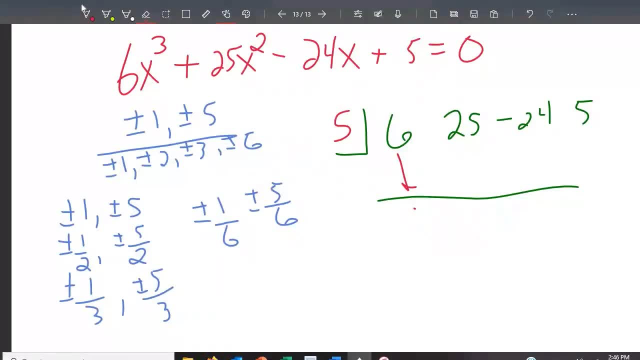 So let's go ahead and try negative 5.. Draw 100.. I sure don't want to have to do a fraction. Six times negative 5 is negative 30.. That gives me negative 5.. Negative 5 times negative 5 is 25.. 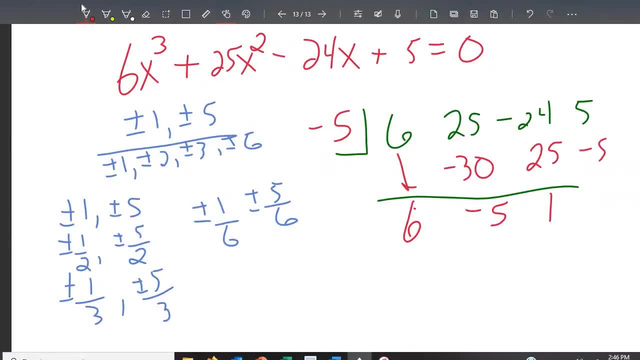 Gives me 1.. 1 times negative 5 is negative 5, and I get 0.. Ooh, thank goodness, That means that's one of my answers. Put the variables back with the coefficients And then we're going to factor this and solve. 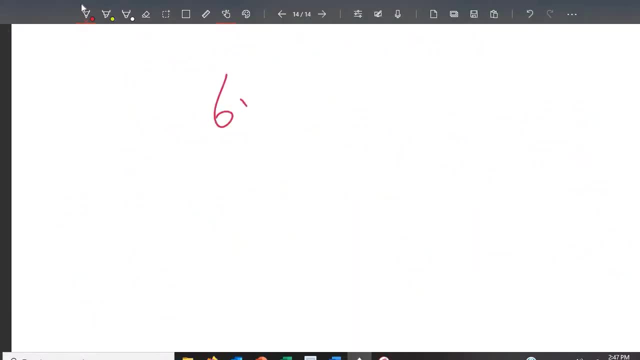 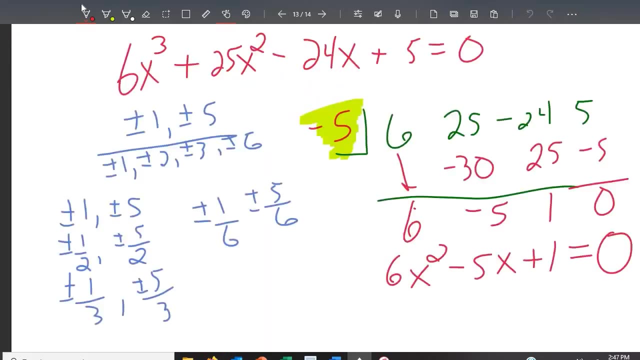 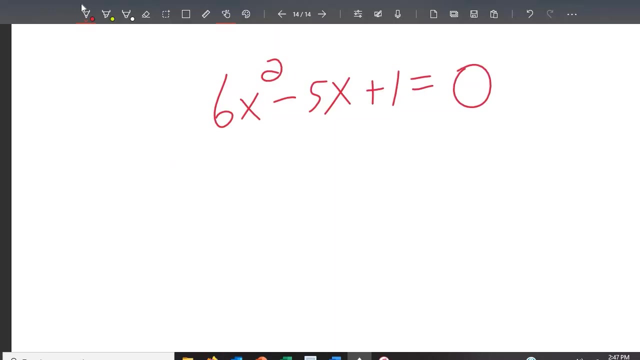 I'm going to come over here on the last slide: 6x squared minus 5x plus 1 equals 0.. Now I want you to factor this Factor and solve, And then I want you to e-mail me your answers for extra points. 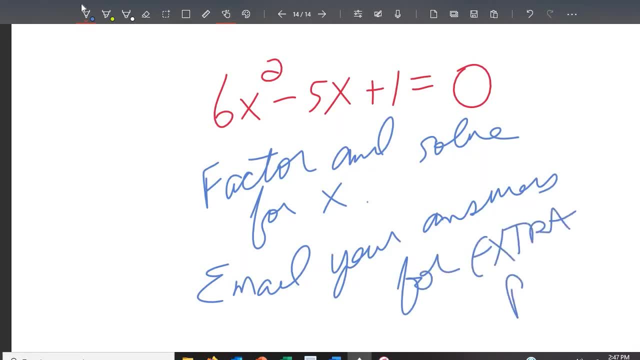 I want to see who's actually doing these lectures.